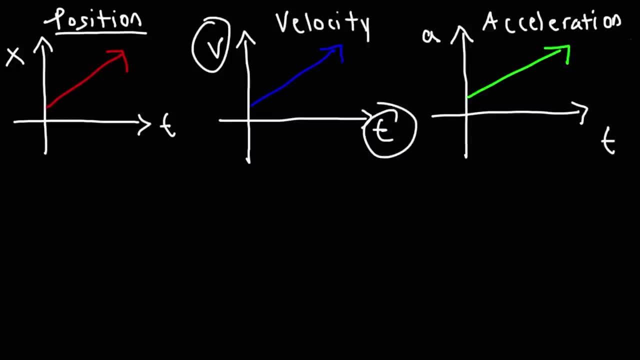 A versus T is the acceleration time graph. Now, what do you think the slope of a position time graph represents? Remember, slope is the change in Y over the change in X. You're dealing with division. So if we were to divide the position or the change in position, 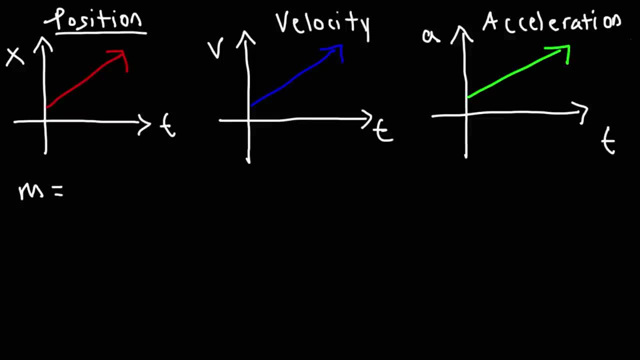 by the change in time graph, we're going to have X versus T. So if we were to divide the position or the change in position by the change in time graph, what will we get? The change in position divided by the change in time. 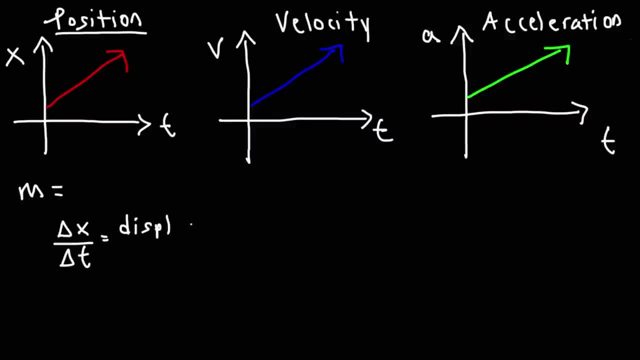 The change in position is displacement. If you divide displacement, Let me just put D for displacement instead of writing everything out. But if you were to divide displacement by time, you're going to get the velocity. So the slope of a position time graph represents the velocity. 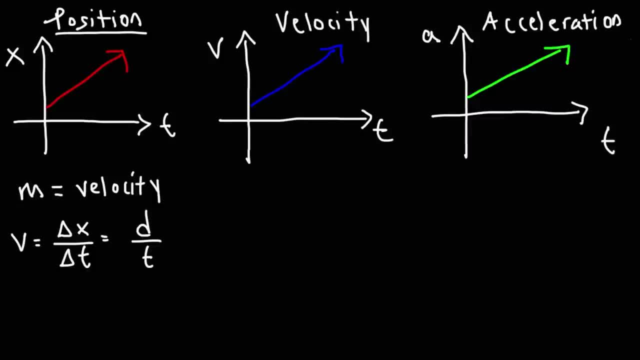 or the instantaneous velocity. If you calculate the slope, let's say like, at a tangent, you're going to get an instantaneous velocity. If you calculate the slope using two points, you're going to get an average velocity. By the way, calculating the slope at one point, 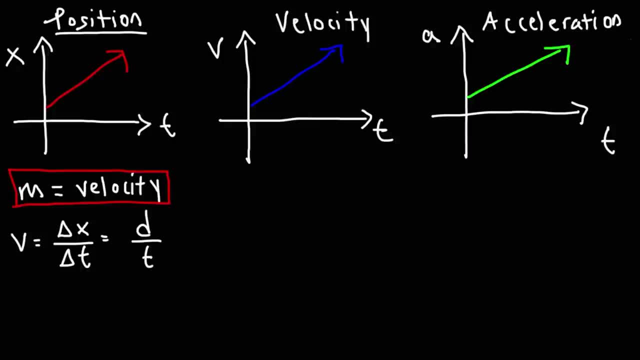 is like finding the slope of the tangent line. That will give you the instantaneous velocity. Calculating the slope using two points, which is the slope of the secant line. that will give you the instantaneous velocity. That will give you the average velocity. 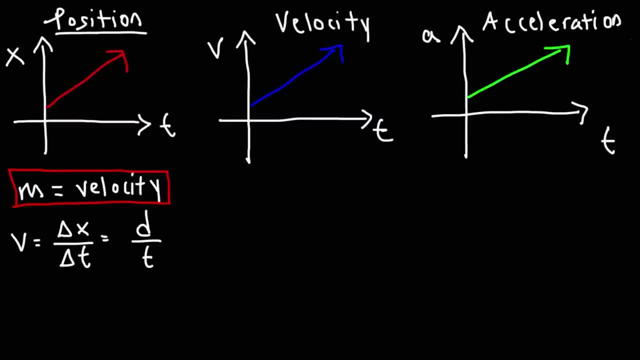 Nevertheless, the slope of the position time graph gives you velocity, So make sure you understand that. Now you might be wondering: what does the area of a position time graph tell us? The area doesn't tell us anything. Remember, area is associated with multiplication. 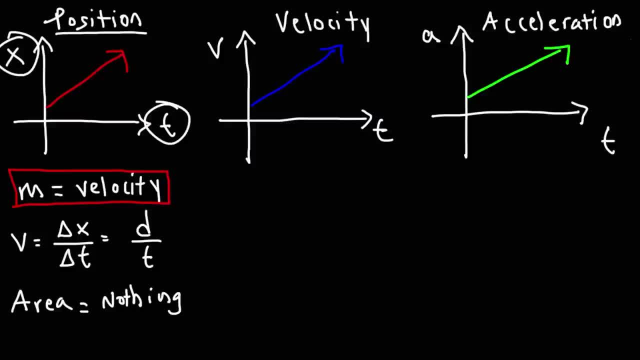 If we were to multiply the y-axis by the x-axis, in this case the change in x by the x-axis, divided by the change in t, we would get meters times, seconds, which it really doesn't help us in physics. So the area for position time graph is not really helpful. 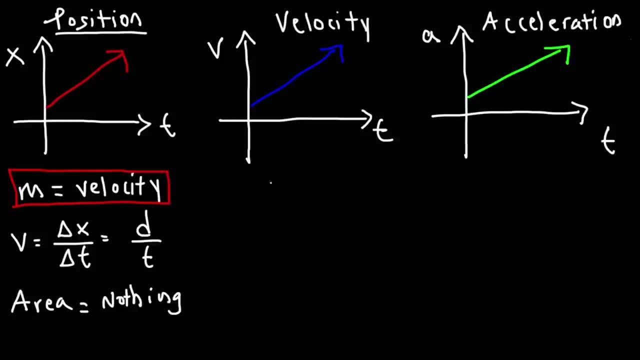 Now, what about the velocity time graph? What does the slope tell us? Well, in order to find out the slope of velocity time graph, we need to use division. If we were to divide v by t, if we were to take the change, 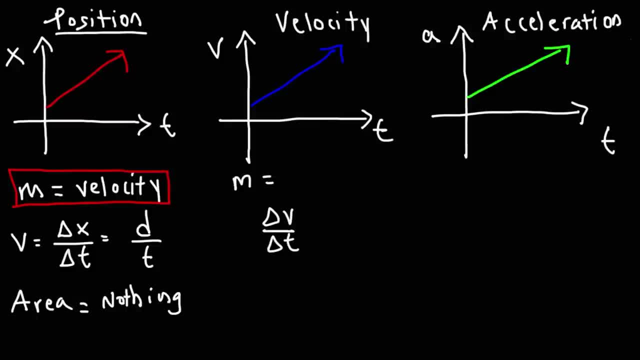 in velocity and divide it by the change in time, what will we get? Velocity typically has the units meters per second and time is usually in seconds. When you divide these two, you get the units meters per second squared. What variable or term is associated? 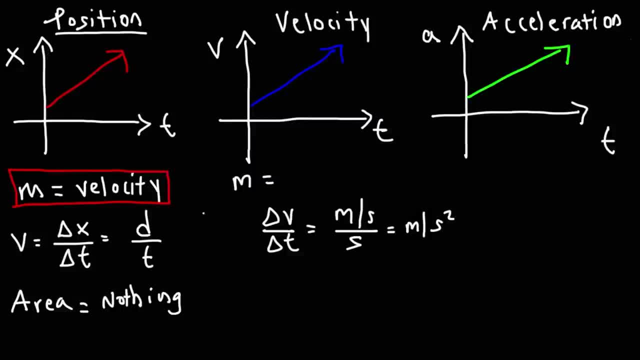 with the units meters per second squared. From physics, you've likely seen it as acceleration. The slope of a velocity time graph is the slope of a velocity time graph is the acceleration. So that's what you need to know when dealing with a VT graph. 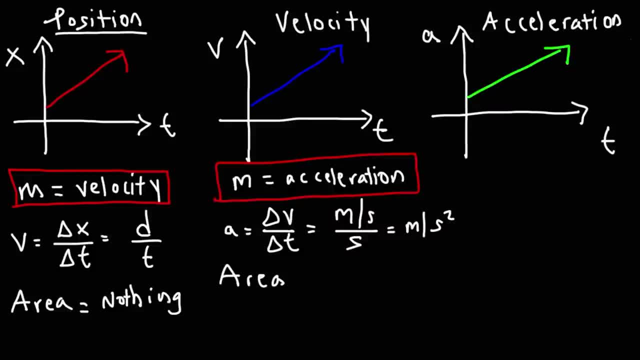 Now, what about area? What does the area of a velocity time graph tell you? So, once again, when you think of area, think of multiplication. If we were to multiply the y-axis by the x-axis, if we were to multiply v by t, 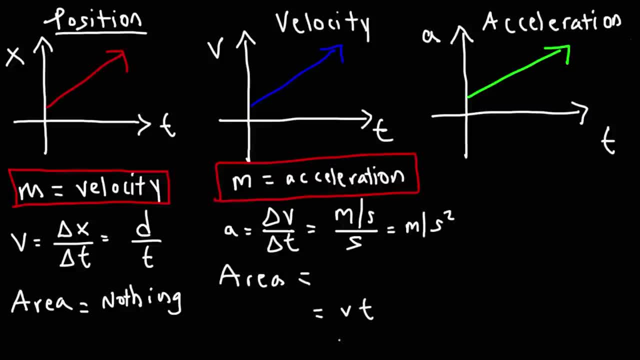 what will we get? Well, let's look at the units. Velocity is usually in meters per second or meters over seconds. Time is usually in seconds. When you multiply these two, the unit seconds cancels, and so we get the unit meters. 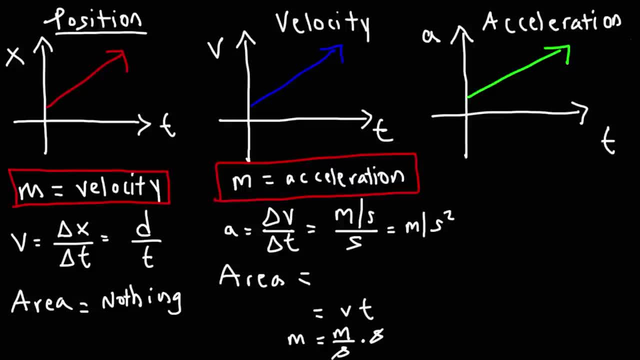 Meters is the unit for distance, position, displacement. But it turns out that when you multiply velocity by time, you get specifically displacement. So I'm going to put this here. So I'm going to put d for displacement: Speed multiplied by time is distance. 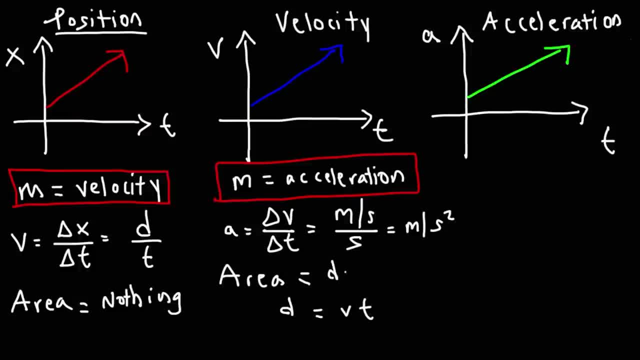 but velocity times, time is displacement, So the area of a velocity time graph is specifically displacement. So when dealing with a velocity time graph, the acceleration- I mean the slope- and the area is important. The slope is the acceleration, the area is the displacement. 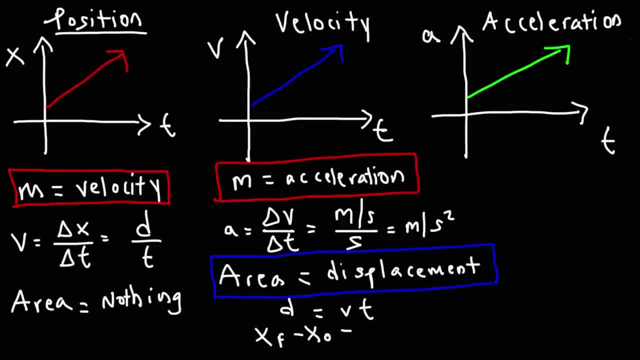 Displacement is the final position, the area and the displacement, So the acceleration is the initial position minus the initial position. If you move this term to the other side, you're going to get this familiar equation: X final is equal to X initial plus VT. 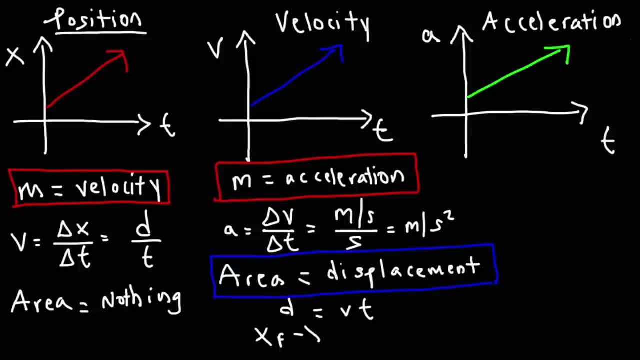 Let me erase that, because I'm going to need the space on the right side. So hopefully you're taking notes or writing these things down, because we're going to use this later in the video. Now let's move on to the acceleration time graph. 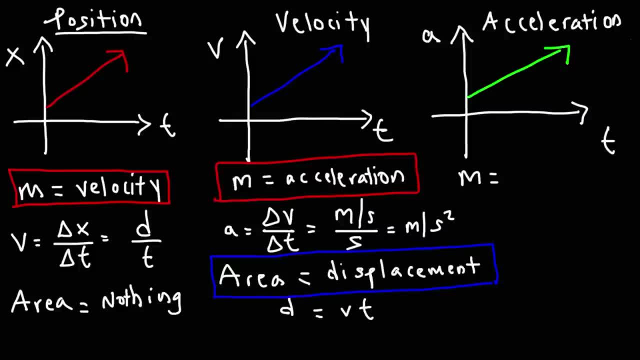 What does the slope, the acceleration time graph and the acceleration time of an AT graph represent? Well, let's divide Y by X. So on the Y axis we have acceleration, on the X axis we have time. So what is the rate of change of acceleration? 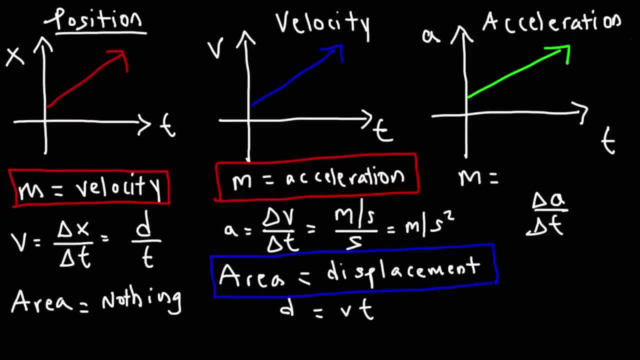 Now for most physics classes that you're going to encounter. you're not going to have to worry about it. This is not going to be applicable to the everyday common situation, But some physics course they do have a value for this, And this represents jerk or jolt. 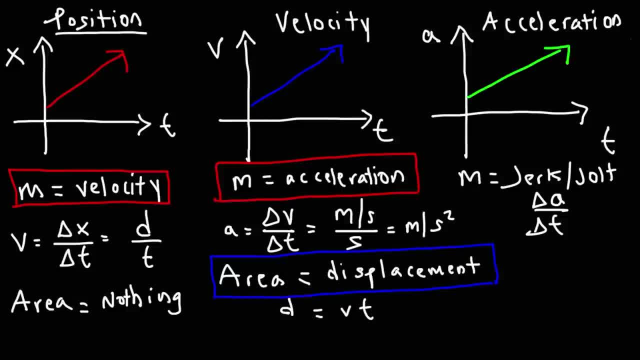 You can look this up on Wikipedia. You may see it in some textbooks, But that's the slope of an acceleration time graph On a physics test. if you're asked the question, what is the slope of an acceleration time graph? and you don't see jerk or jolt? 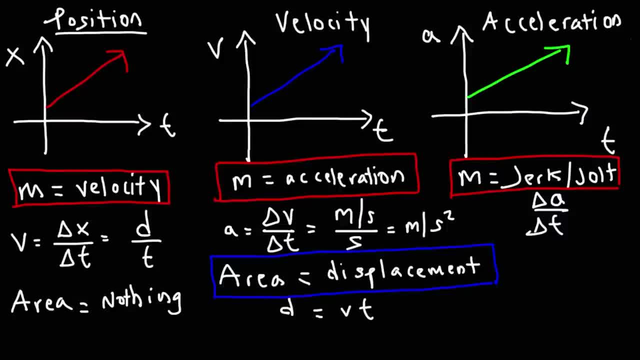 you might have to go with nothing, because maybe your teacher didn't cover that topic, Because for most physics course you won't see this. But in the event that you do see those terms, that's what it is. Now, what about the area of an acceleration time graph? 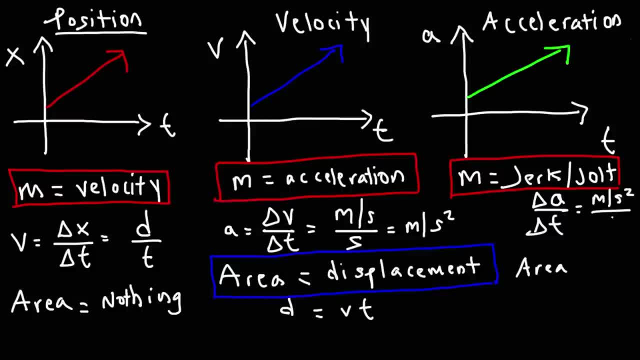 By the way, the units for this would be meters per second squared over seconds, So it would be meters per second cubed. So that tells you you're dealing with the rate of change of acceleration. By the way, the rate of change of position. 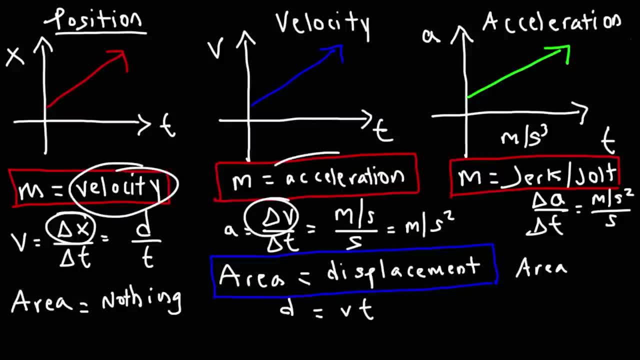 is velocity, The rate of change of velocity is acceleration, And the rate of change of acceleration, as we just mentioned, is jerk or jolt. Now for the area: we're multiplying Y by X, In this case acceleration by time. 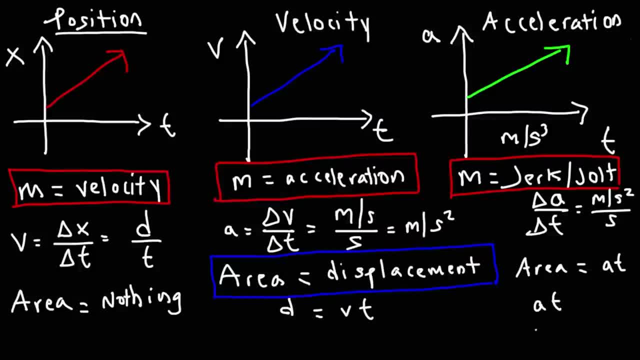 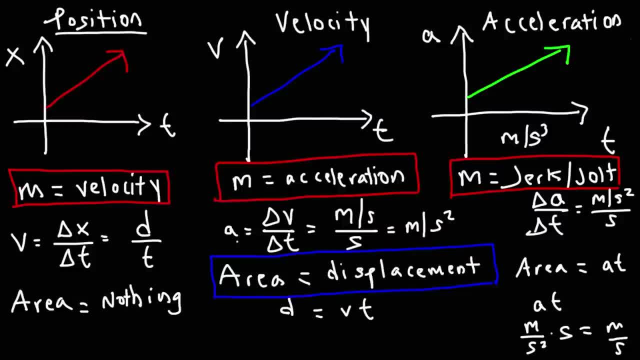 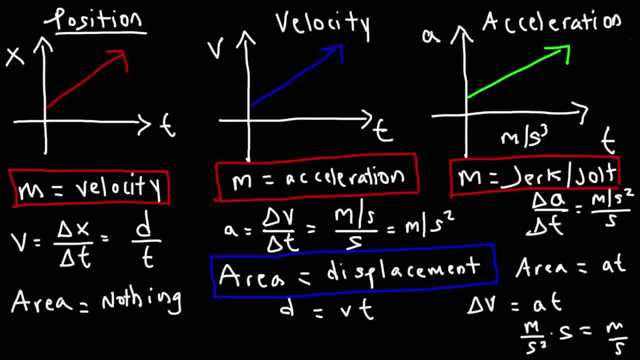 So A times T gives you the change in velocity. If you replace delta V with V final minus V initial, you get this familiar equation: V final is equal to V initial plus A T. So the area of an acceleration time graph is the change in velocity. 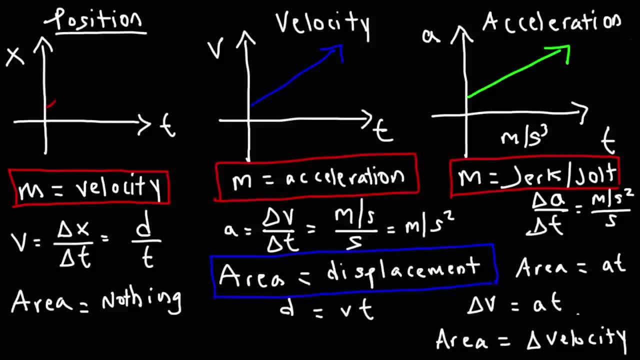 Now let's qualify that statement. So let me change this graph real quick. So let's say we have a curve that looks like this, Let's say that's our position time graph And let's put some numbers. Let's say this is one, this is three and this is five. 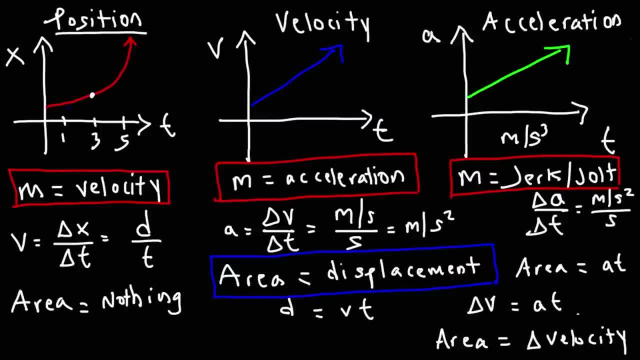 So let's say that's our position. time graph. So let's say that's our position time graph. Now, if we draw a line at three, a line that touches the curve at one point, my lines are terrible. let's do this one more time. 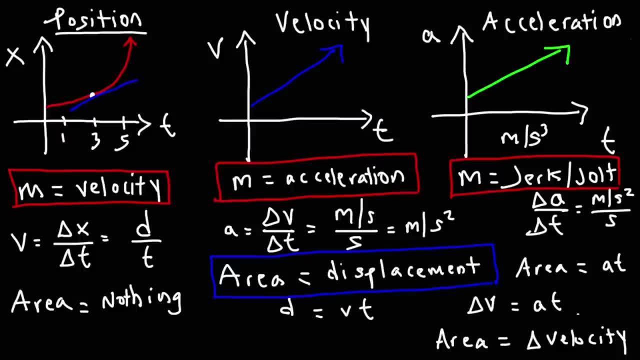 I will make the best of that. But a line that touches a curve at exactly one point, that line is known as the tangent line. The slope of a tangent line gives you the instantaneous velocity if you're dealing with a position time graph. So let me say that one more time. 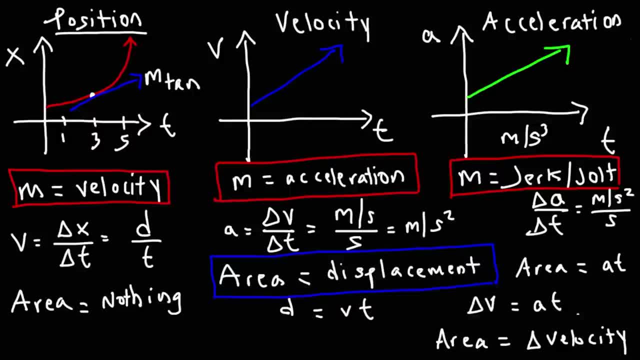 So let me say that one more time. The slope of the tangent line of the position time graph gives you instantaneous velocity. That is the velocity instantly when t is equal to three seconds. Now let's say, if we have two points at one and five. 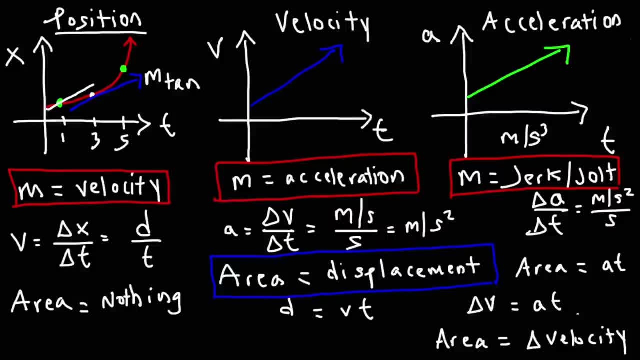 And let's draw a line connecting those two points, A line that touches the curve at two points. that line is a secant line. A secant line gives you the average velocity. The slope of the tangent line gives you the instantaneous velocity. 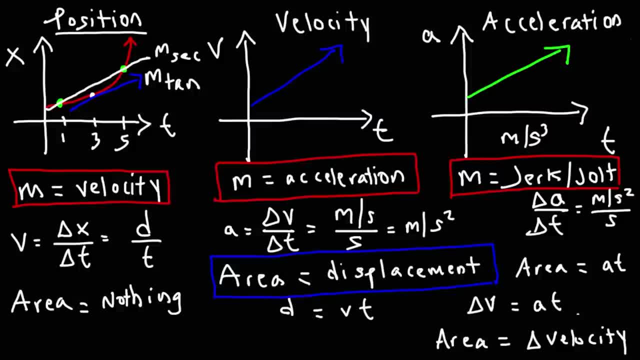 To calculate the instantaneous velocity. that's a little difficult because it's hard to find the slope at one point. Now you could use calculus, You could find the derivative and that can give you the slope of the tangent line, which is the instantaneous velocity. 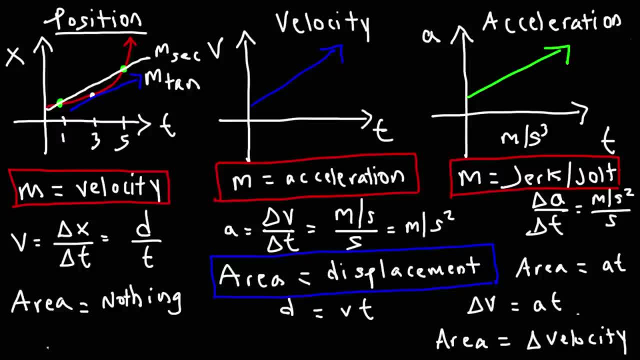 The slope of the secant line. you could use algebra to get that answer. You could use y two over y one divided by x two minus one. So it's easy to find the slope of the secant line, which is the average velocity. 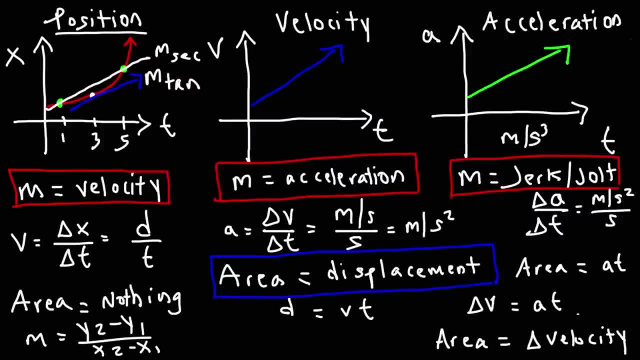 Now you can approximate the slope of the tangent line using the slope of the secant line. So if we want to get a good estimate of the slope at exactly, t equals three, if we know what the position is at, let's say 2.9 and 3.1,. 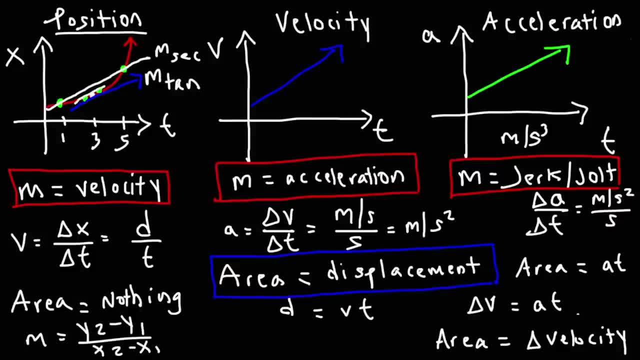 we can calculate the slope of the secant line of those two points- 2.9 and 3.1, to approximate the slope of the secant line. So we'll approximate the slope of the tangent line at three, The closer those two points get to three. 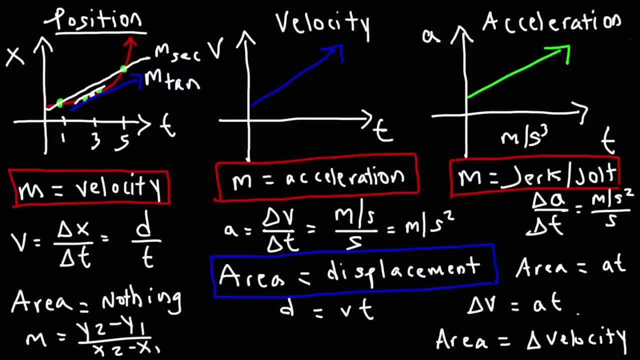 the more accurate the secant line becomes to the slope of the tangent line. So as those two points get closer and closer to three, the slope of the secant line approximates the slope of the tangent line. So that's how you can find the slope of the tangent line. 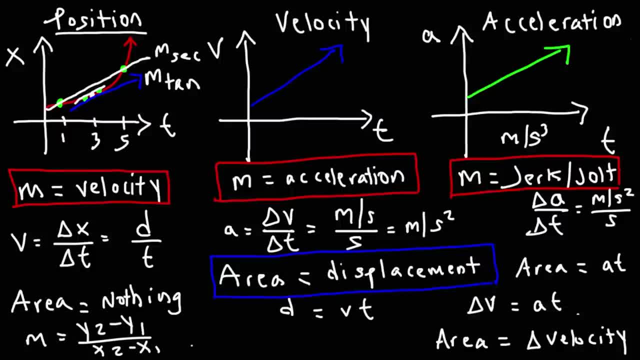 using this formula. So if you were to use values like 2.99 and 3.01, it's gonna be a very accurate estimate of the slope of the tangent line. So let's put this all together When dealing with a position time graph. 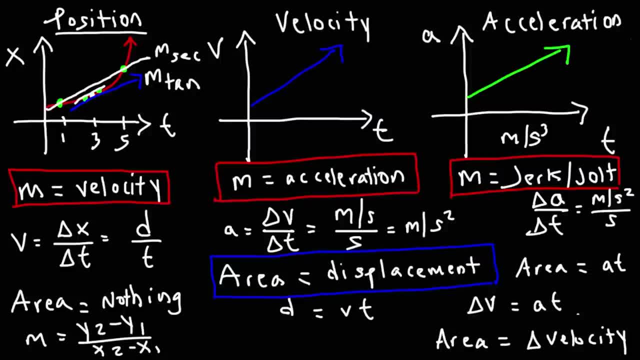 the slope of the tangent line gives you the instantaneous velocity. The slope of the secant line gives you the average velocity. When dealing with an acceleration time graph, the area doesn't give you the instantaneous velocity, nor does it give you the average velocity. 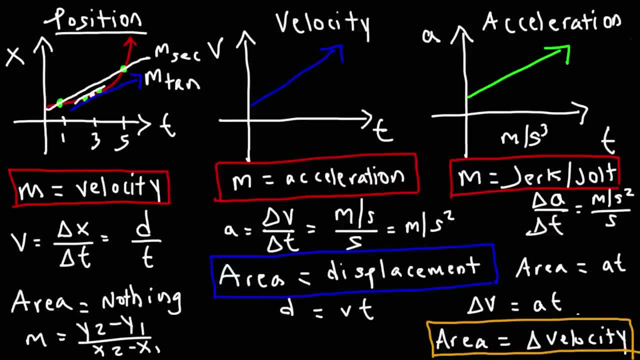 but it gives you the change in velocity That is v final minus v initial. So just make sure you see that distinction. So that's the first step. The second step is the distinction. And remember the slope of a position time graph is velocity. 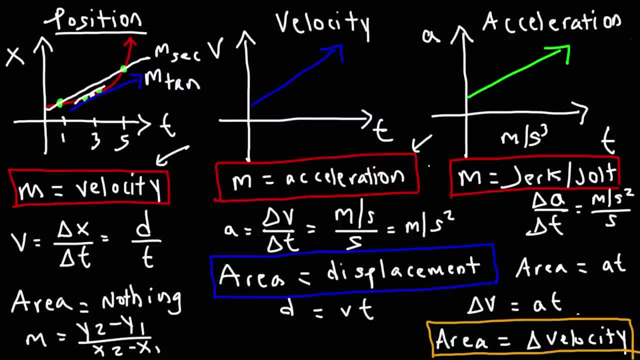 The slope of a velocity time graph is acceleration. The slope of an acceleration time graph is jerk or jolt, which is not commonly used, And the area of a velocity time graph is displacement. The area of an acceleration time graph is velocity. Those are things you have to know. 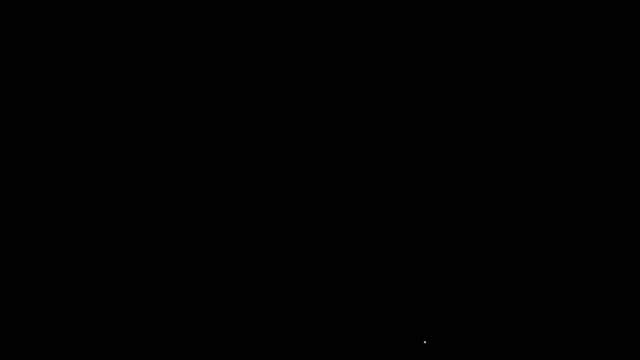 if you wanna answer questions with these time graphs. Now I'd like to make a distinction. Let's make a distinction between two similar time graphs: A position time graph and a distance time graph. In physics, position time graphs, you'll typically see them as x versus t. 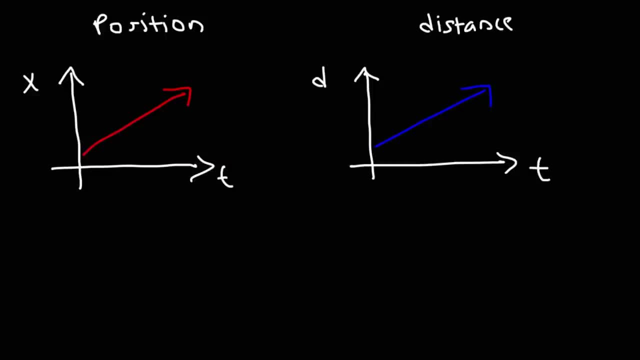 For a distance time graph. you'll see them as d versus t. Now what you need to know is that velocity, which I'll just put v velocity, is displacement over time. Speed is equal to the distance divided by the time. So here we're dealing with division. 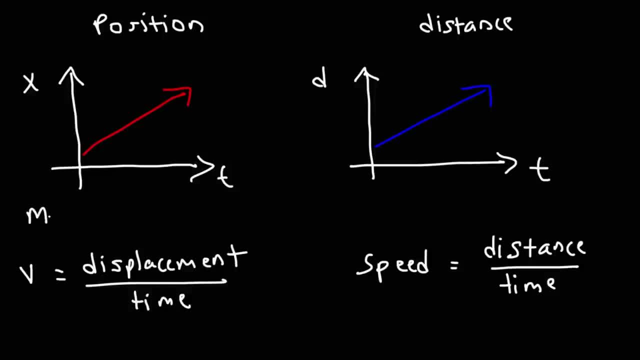 So think of division as slope. The slope of a position time graph is velocity, But the slope of a distance time graph is speed, Because, remember, the slope is d over t, distance over time, which is speed. So that's the difference between a distance time graph. 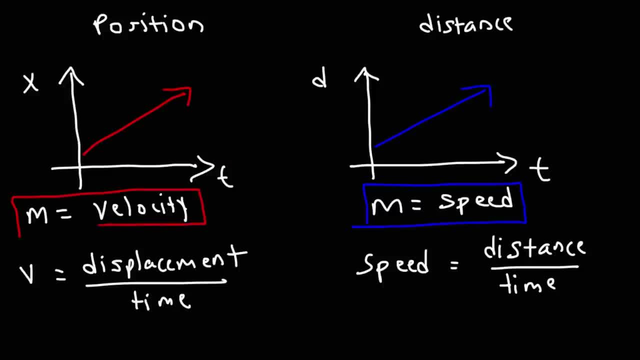 and a position time graph. The position time graph can give you velocity if you calculate its slope, but a distance time graph- let me make sure I said that correctly- a position time graph- can give you the velocity if you calculate the slope. 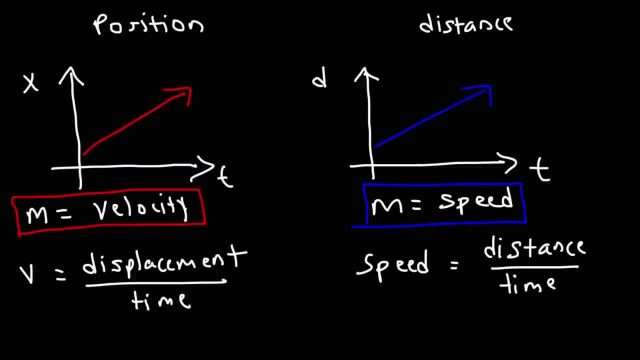 but the distance time graph can give you the speed if you calculate the slope. So remember, velocity is a vector and speed is a scale of quantity. Velocity can be positive or negative, but speed is always positive. So make sure you see the difference between the two. 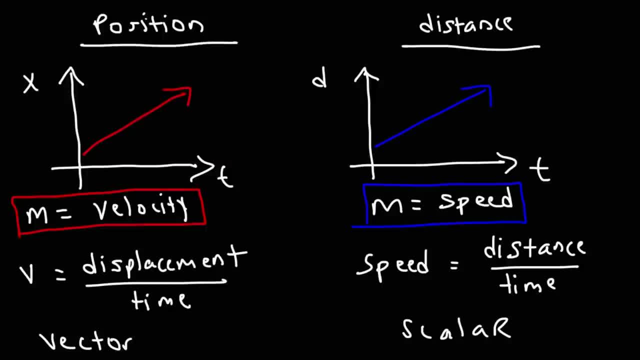 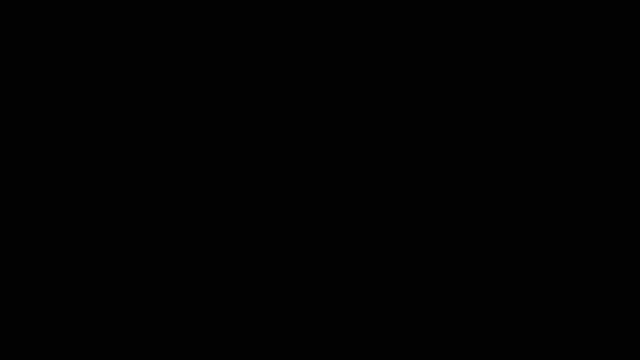 if you're dealing with a position time graph versus a distance time graph. Now let's take some more notes. So we said that velocity is. So we said that velocity is the rate of change of position. Therefore, as the position increases, 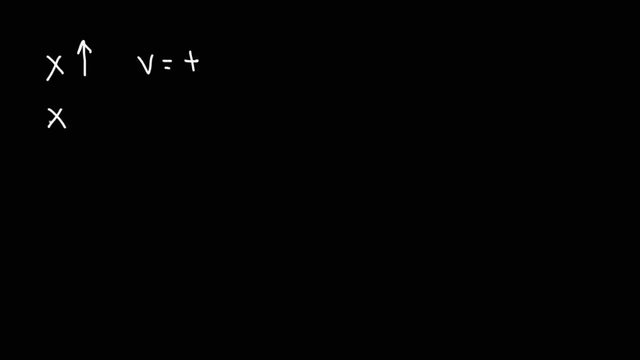 the velocity is positive. When the position is decreasing, velocity is negative. So if x is going up, that means that the particle or the object is moving to the right along the x-axis. If x is going down, that means it's moving to the left. 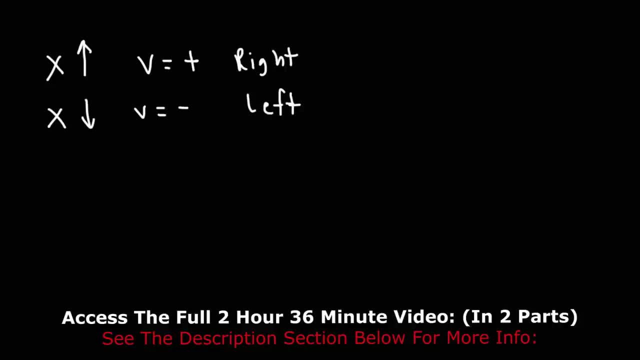 So any time velocity is positive when you're dealing with an x versus t graph, that means the particle is moving to the right. If velocity is positive, that means it's moving to the right. is negative, it's moving to the left. If the position is constant, that means the 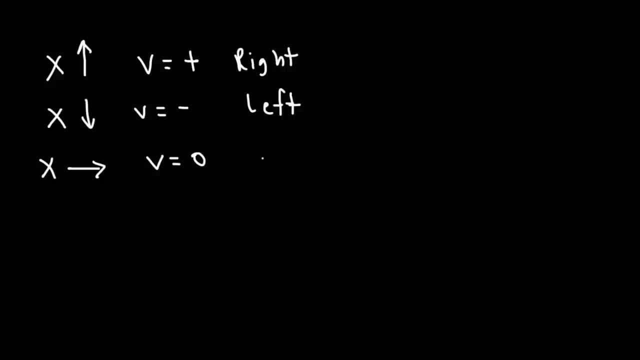 velocity is zero. Now, when the velocity is zero, it could be that the object is at rest, or it could be that the object is changing direction. So it really depends on the shape of the graph. So, for instance, let's say: if you have a 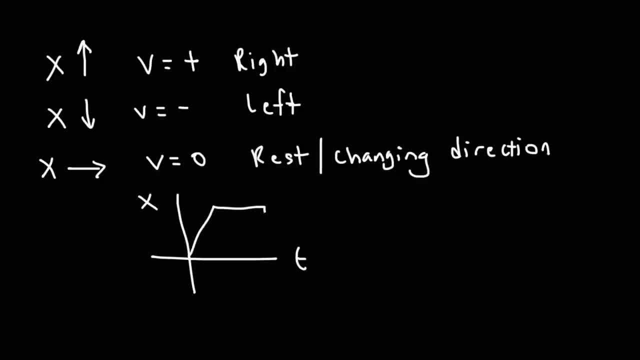 position time graph that looks like this. so notice that it's horizontal for quite some time. at that moment, the particles at rest, but it could change instantly. let's say, if it looks like this, Well, let's do it like this actually. so notice that it's horizontal for a very 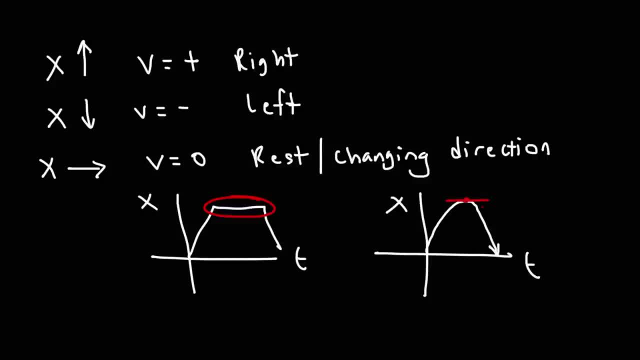 brief moment, the tangent line, which is the slope. at that one point the slope of that tangent line is zero, because the line is horizontal and so at that instant it's at rest. but it's changing direction. so here the position is increasing. that means the particles moving to the right, because the slope is 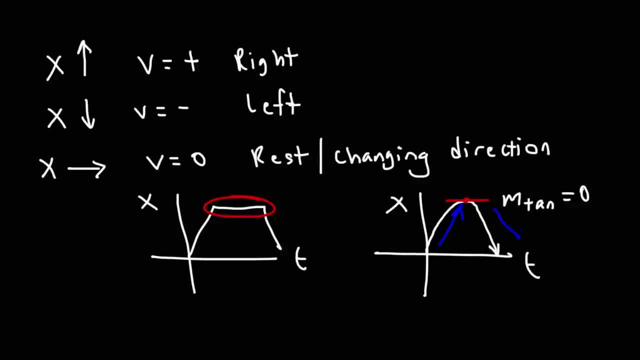 positive, those velocities positive. here it's going down. that means the slope is negative, which means velocity is negative. so it's moving to the left. so it was moving to the right and now it's moving to the left. so at the top, at that peak where the slope is zero, it's at rest for a very, very short time or more. 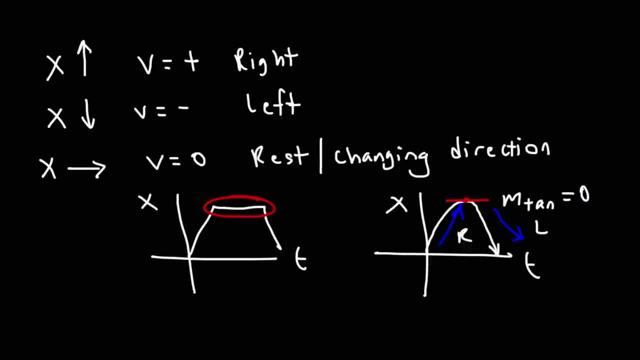 specifically, it's changing direction, going from right to left. so when velocity is zero, the particle could be at rest, and then it's moving to the right, and now it's moving to the left. so at that peak, where the slope is at rest for a very, very short time, or the particle 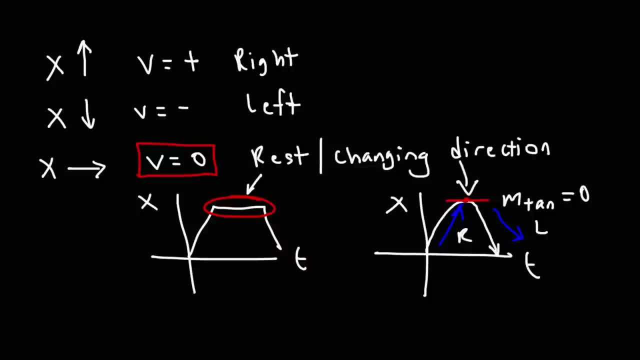 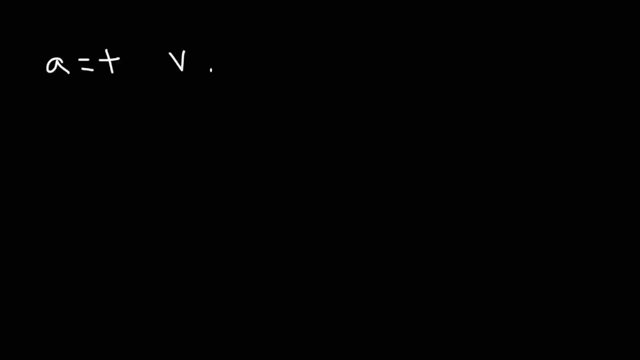 could be changing direction. so keep that in mind. now, we said that velocity is the rate of change of position. acceleration is the rate of change of velocity, so whenever the acceleration is positive, that means that the velocity is increasing. when the acceleration is negative, the velocity is decreasing. if 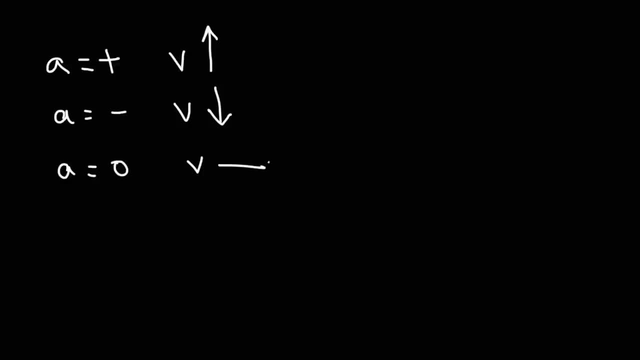 the acceleration is zero, that means that the velocity is constant. now, speed is the absolute value of velocity. so if the velocity is positive- 5 meters per second- that means that the speed is positive 5. if the velocity is negative- 4 meters per second- that means that the speed is. 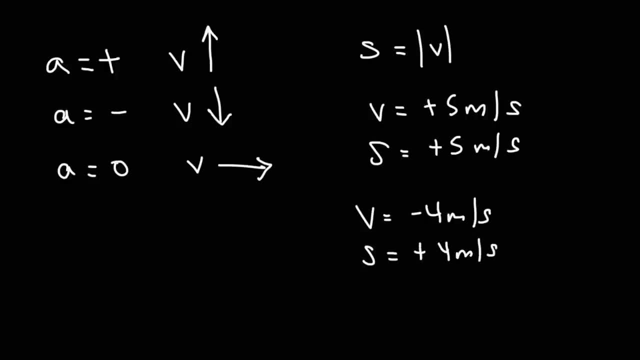 positive 4 meters per second. so if a particle is moving to the left at 4 meters per second, you would say that the speed of the particle is simply 4 meters per second. speed is always positive. now we need to talk about when an object is speeding up versus when it's slowing down. how can you determine? 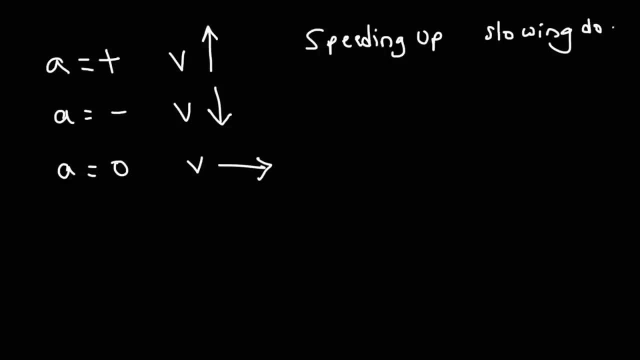 when it's speeding up and when it's slowing down. here's a quick and simple way to determine the velocity of the particle, when it's speeding up and when it's slowing down. here's a quick and simple way to get the answer. a particle is speeding up when the acceleration and velocity. 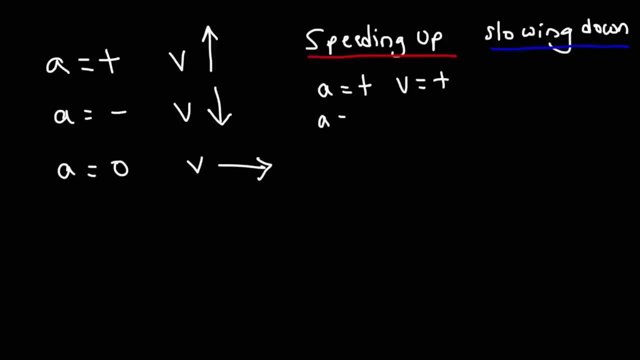 have the same sign: either they're both positive or both negative. in this situation, the velocity is increasing. it's becoming more positive because the acceleration is positive here, even though the velocity is negative, it's becoming more negative, and so if you get a larger negative, the speed, which is the 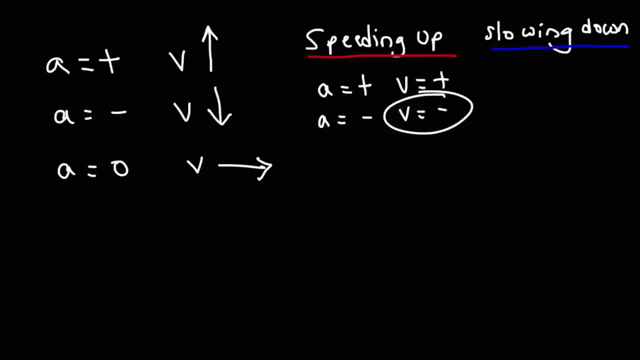 absolute value of velocity that's becoming more positive. so in both cases it's speeding up. when the signs of acceleration and velocity are different, where one is positive and the other is negative, that's when the particle or the object is slowing down. so let's think about this conceptually here. when the 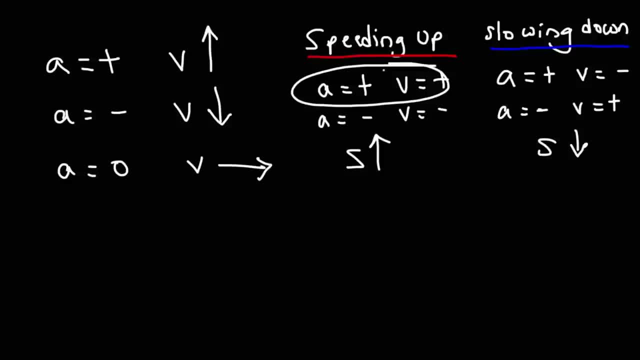 acceleration is positive, that means velocity is increasing, velocities becoming more positive, which means speed is becoming more positive. so speed is increasing, the acceleration here is negative and the velocity is negative. because the acceleration is negative, the velocity is becoming more negative. so think of it as going from negative 5 to negative 8, but speed being the absolute. 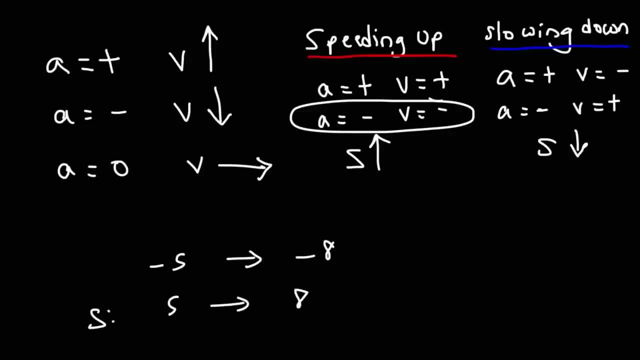 value of velocity. it's going from 5 to 8, so speed is increasing. in that case, now for this situation: the velocity is negative, but the acceleration is positive, which means that the velocity is becoming less negative. so to illustrate this, let's say if the velocity was negative, 5 acceleration is. 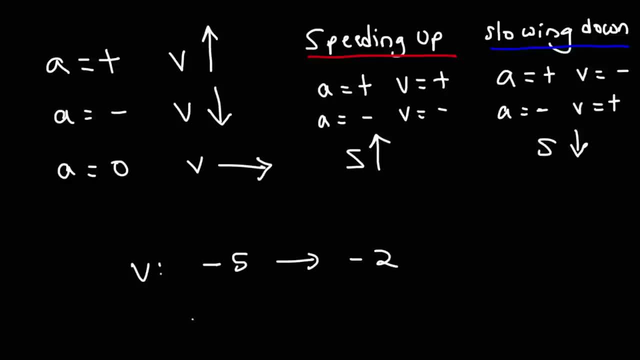 making it less negative, more positive, so it would become like negative 2. due to a positive acceleration, the velocity is increasing when acceleration is positive. so negative 2 is higher than negative 5 on a number line. but if you take the absolute value of it, you can see why the speed is decreasing, going from 5 to 2 S. 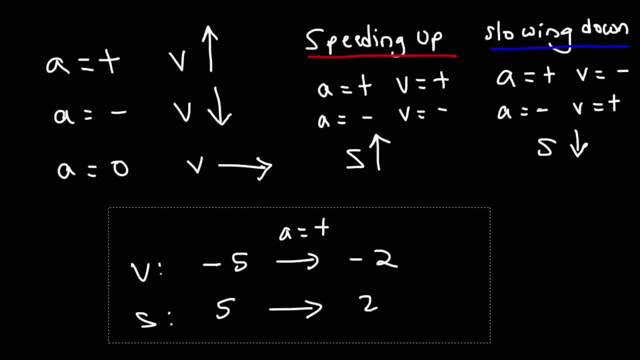 slowing down. now a quick illustration for the last one: where acceleration is negative but velocity is positive, the velocity is becoming less positive. so let's say, if, what if was 8 with a negative acceleration, it can go down to 4. speed being the absolute value of velocity will be the same going from 8. 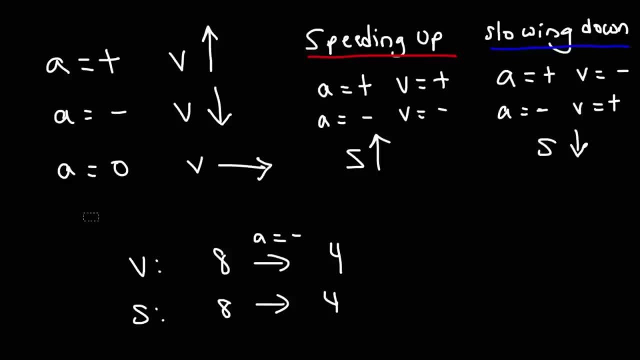 to 4, so the speed will be decreasing. thus, any time an object is slowing down, the acceleration and velocity have opposite signs. when it's speeding up, the acceleration and velocity have the same sign. so that's a quick and simple way to determine if an object is speeding up or if it's slowing down. now let's focus on 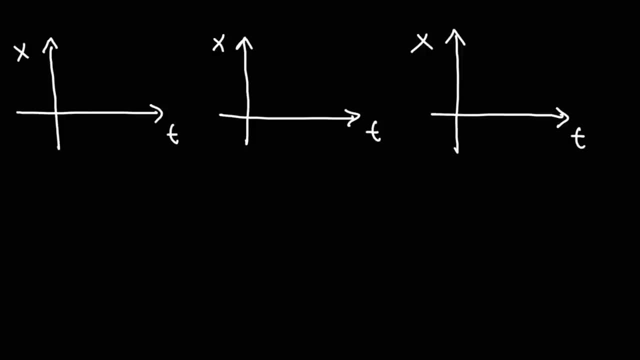 the three linear shapes of a position time graph. now these linear shapes exist for any graph, so you can have a straight line going up, you could have a straight line going in a horizontal direction or a straight line going down. those are the three linear shapes that you're going to be dealing with now. 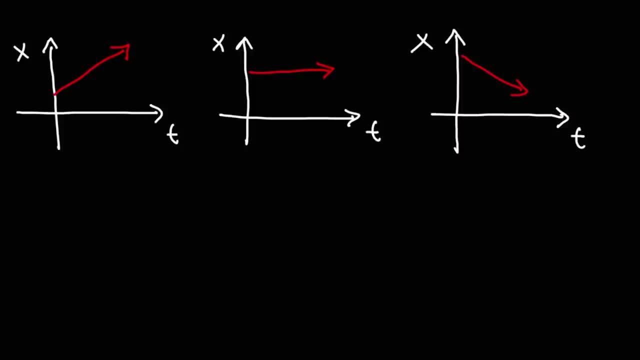 because these shapes are linear, the slope is constant and for position time graph, velocity is the slope. so for these three situations, velocity is constant. and when velocity is constant, what can you say about acceleration? anytime velocity is constant. acceleration is zero is zero for each of these three position time graphs. Now for the first one, the 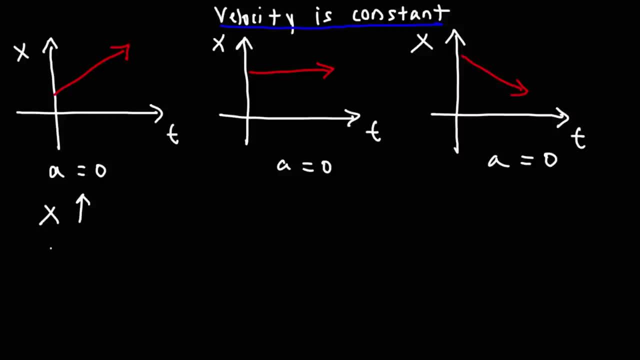 position is increasing. Anytime the position is increasing, the velocity is positive. For the second one, the position is not increasing, it's constant. so the velocity is at zero, which means it could be at rest or it may be changing direction. But for this particular shape here it's at rest, It's not changing. 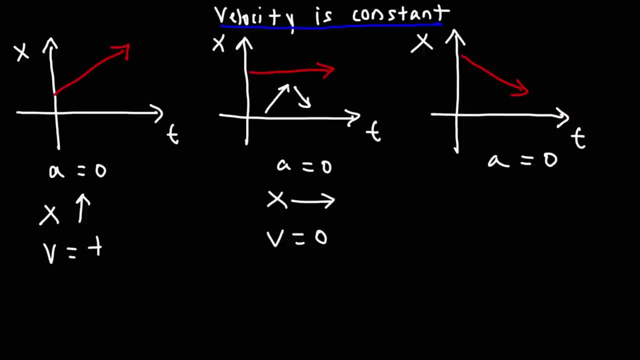 direction. It's not going up and then down. But when V is zero, if you don't have the graph, just know that it could be at rest or it could be changing direction. Here the position is decreasing. Whenever the position decreases, the velocity is negative. So when dealing with a position time graph, 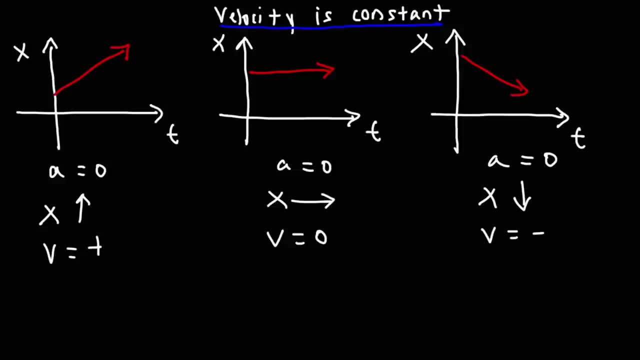 if you have these three shapes, just know acceleration is zero. If it's going up, velocity is positive. If it's going down, velocity is negative. If it's horizontal, velocity is zero. So in this side it's moving to the right Along the x-axis, here it's moving to the left And for. 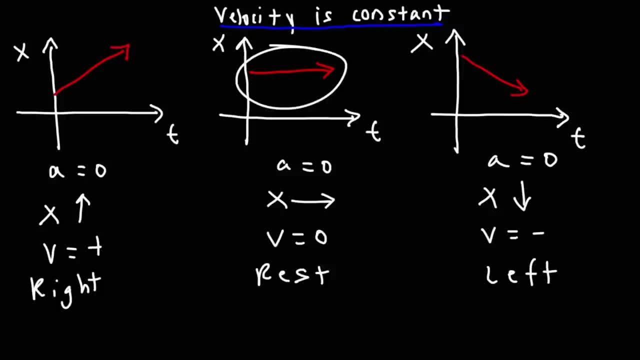 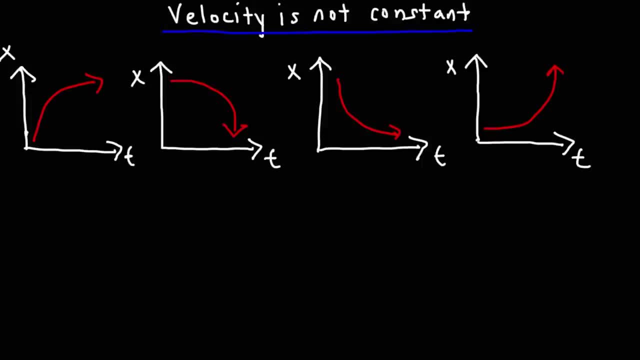 this particular picture, specifically this one. it's at rest. Now let's consider the next four fundamental shapes that you'll see with a time graph. So now we don't have the three linear shapes that we did before, but we have four parabolic. 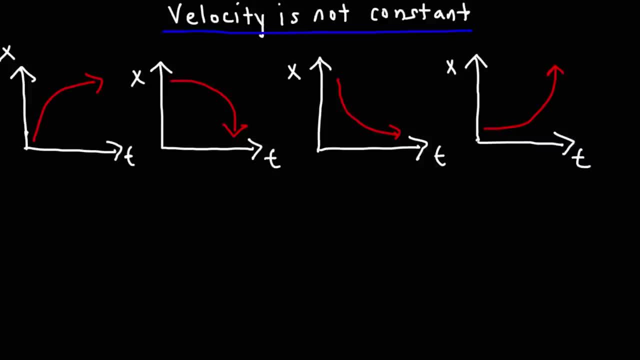 shapes Because the position time graph is not linear, the velocity is not constant. Therefore we have an acceleration. But before we go into acceleration, let's talk about velocity. So for the first one, is the velocity positive or negative? Well, the position is increasing because we're going up along the y-axis. So 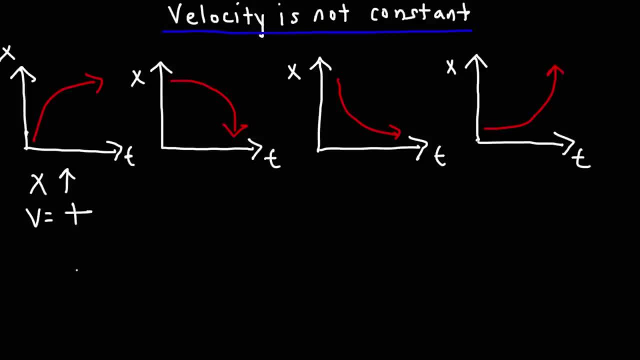 therefore velocity is positive, because the slope is positive. Here the position function is decreasing, So therefore velocity is negative. For this particular shape the position function is still decreasing, because we're going down, So velocity is negative as well. But here we're increasing, So x is going up. 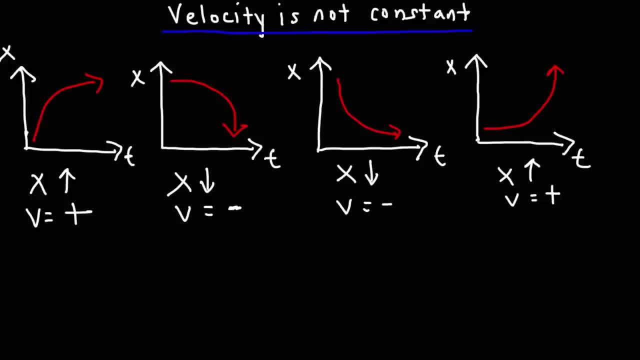 Therefore, velocity is positive. So that's the velocity for each of those four situations. Now what about acceleration In calculus? if you've taken it before, this shape is concave down. This shape is known as concave up When dealing with a position time graph, if you have a, 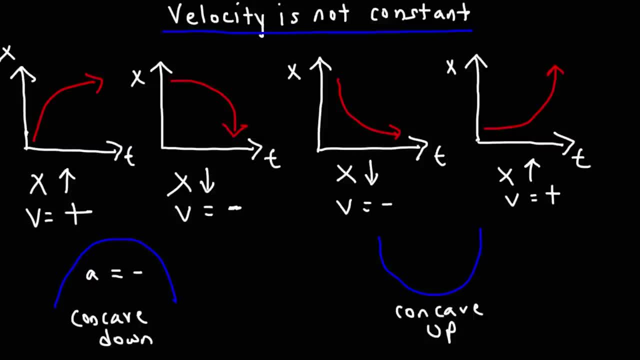 concave down shape. the acceleration is negative, So down for negative and up for positive. So for now, go ahead and write that down. So notice that these two combined form a concave down shape. I put them like that together so you can easily tell that. 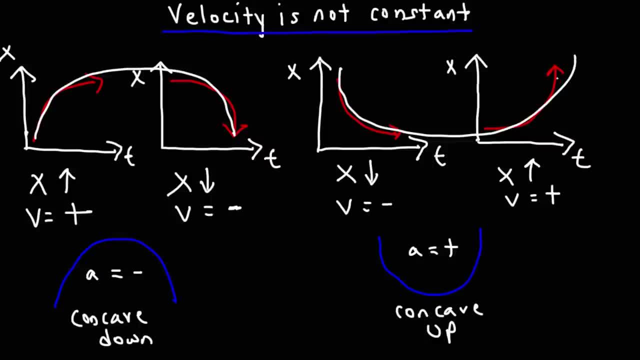 the acceleration will be negative. These two shapes combined form a concave up shape. This is the first half of it and that's the second half. So for the first two shapes acceleration is negative and for the last two acceleration is positive. Now let's look at this from 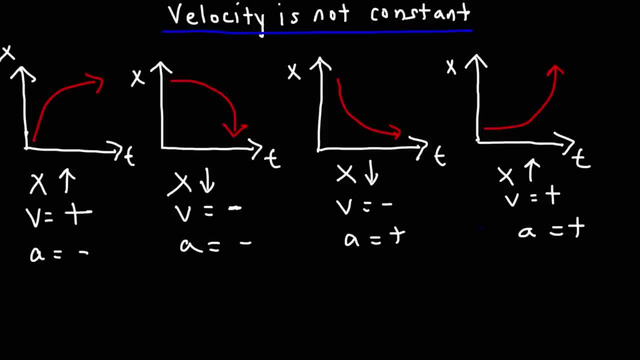 another perspective. We know that the slope tells us the velocity, but the way that the slope changes tells us the velocity, So let's look at this from another perspective. So if we analyze how the slope changes, we can get an idea of the acceleration for this. 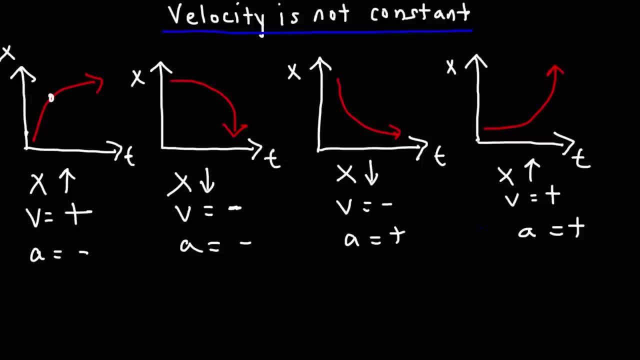 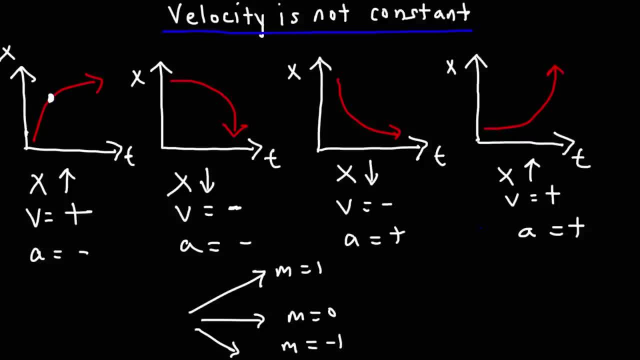 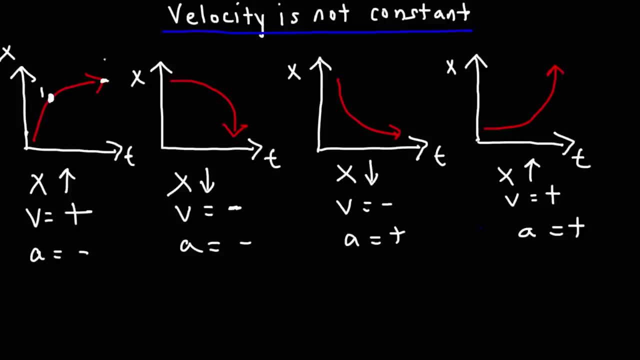 almost horizontal, where the slope is approximately 0. So the slope is going from 1 to 0.. Even though the velocity is positive, because x is increasing, we're going up, we're going down, The slope is decreasing. It's going from 1 to 0.. Therefore, we can see why the 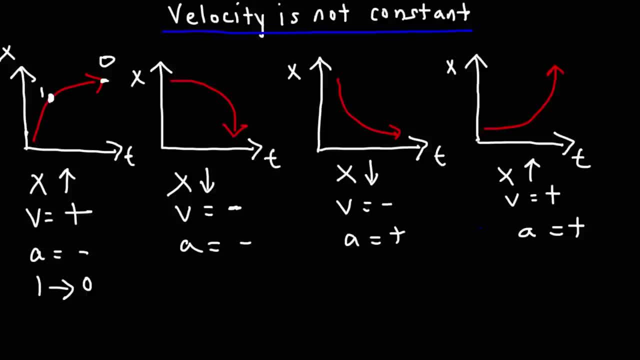 acceleration is negative. Remember, the slope represents the velocity. So if the velocity is going from 1 to 0, it's decelerating. That's why we can say the acceleration is negative. So now let's analyze the slope for the second one. So here it appears horizontal And 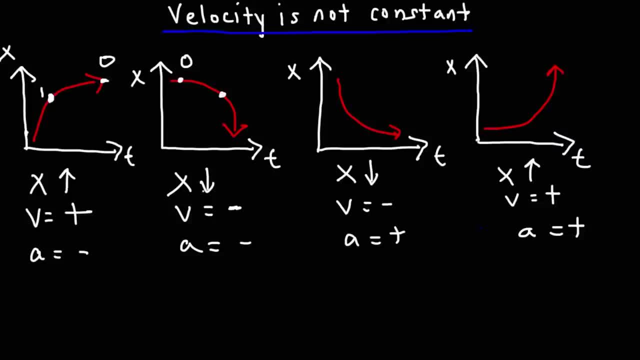 at this point it looks like it's going down at a 45 degree angle. So the slope or the velocity is going from 0 to negative 1.. So it's still decreasing. Negative 1 is less than 0.. So we can see why the acceleration is negative. Let me keep these numbers here. 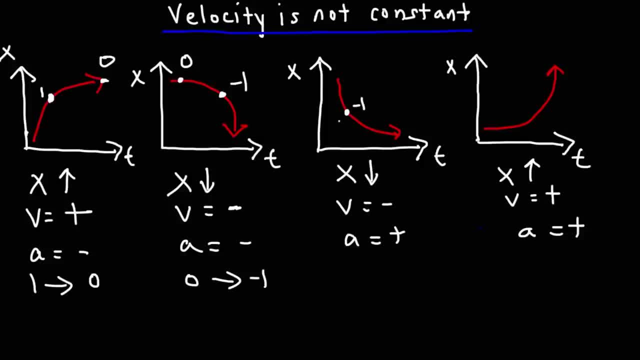 Now, at this point, the slope appears to be negative 1.. It's going down at a 45 degree angle, But it's becoming horizontal where the slope is 0. So going from negative 1 to 0. The slope, or the velocity, is increasing. Thus we can see why the acceleration is positive. 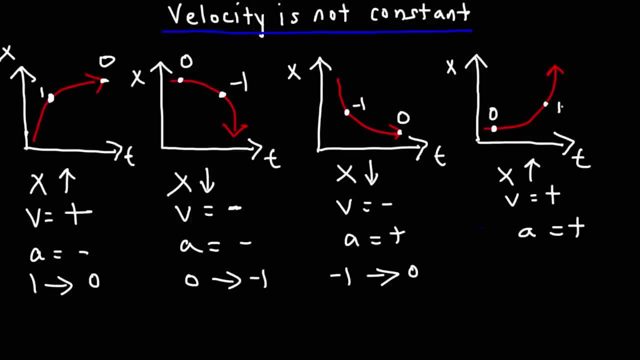 And here it's clear to tell. The slope appears to be 0. And here it's going to 1.. So from 0 to 1, the velocity is increasing, which means the acceleration is positive. So any. 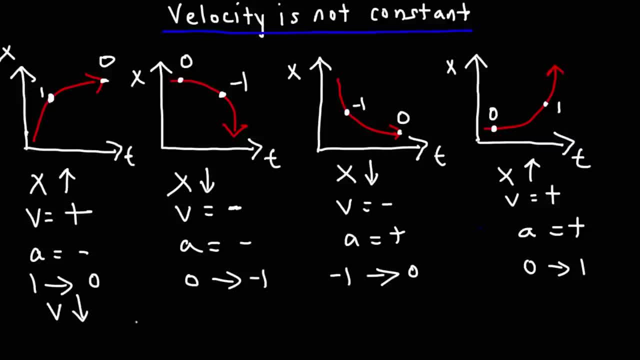 time the acceleration is negative, the velocity is decreasing. When the acceleration is positive, the velocity and the slope is increasing. Now the last thing that we need to talk about is if it's speeding up or slowing down. So looking at the first graph on the left, would you say it's speeding up or slowing. 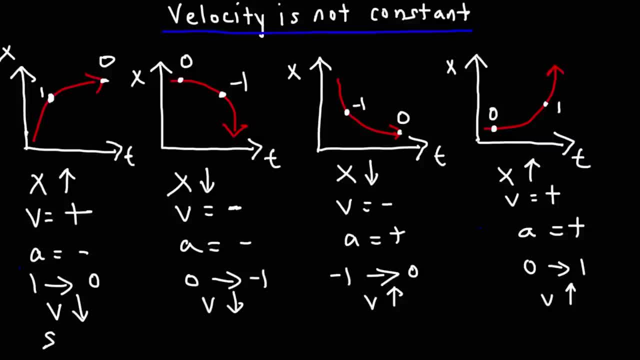 down. So if we look at the signs for velocity and acceleration, they're different, So we can say that it is slowing down. Remember, speed is the absolute value of velocity. If you go from 1 to 0, you're slowing down. 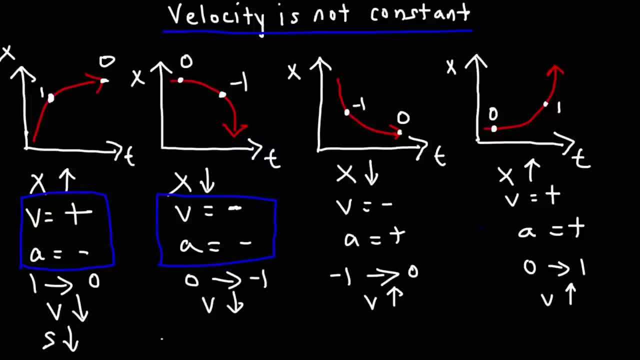 Here the signs are the same. So it's going to be speeding up this time. Velocity is 0.. Speed, being the absolute value of velocity, is not negative 1, but positive 1.. So in this case, the speed is going from 0 to plus 1.. It's speeding up Here. the speed is going.